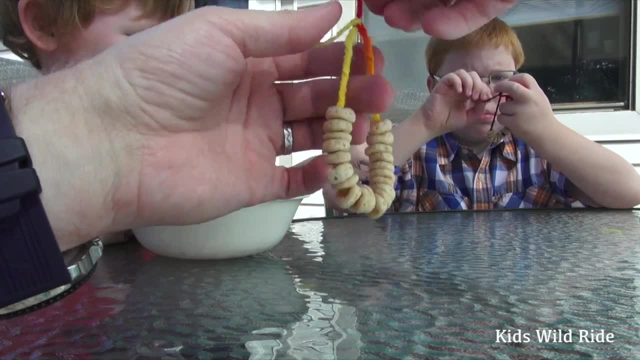 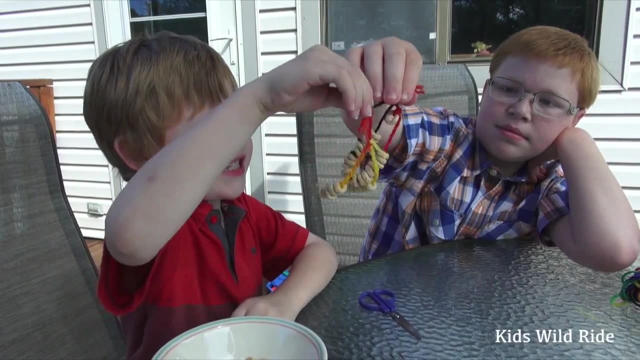 Zippity-doo-dah, There we go. So we have our little feeder And Owen's tying his up. now Cheerio bite. Maybe a squirrel will get one. One more thing we're gonna do now: Hold on, this, is it? 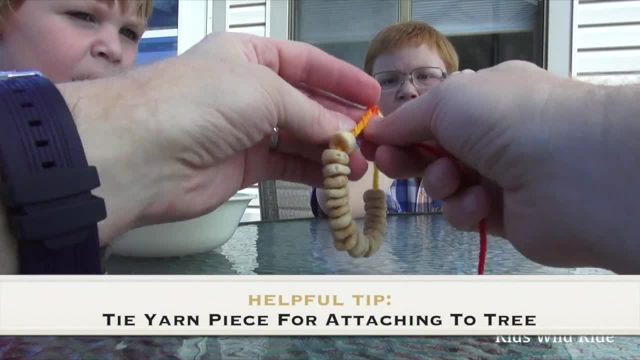 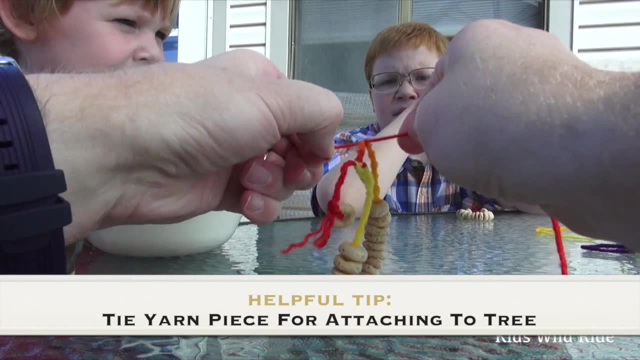 We cut another piece of yarn. We're gonna take it and tie it. Little knot on our Cheerio holder. Little knot on our Cheerio holder. Little knot on our Cheerio holder. Nice secure knot. Nice secure knot, Nice tight one. 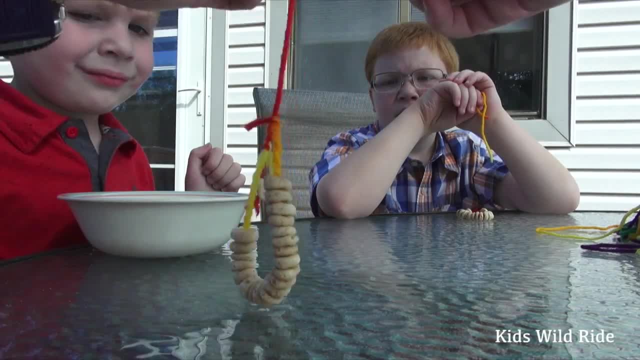 And then we have that part to tie on the branch, And then we have that part to tie on the branch, So we'll do the same to Owen's, And then we're gonna take out and find a tree, And then we're gonna take out and find a tree. 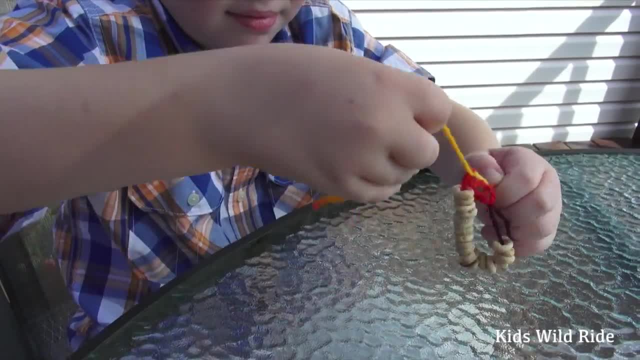 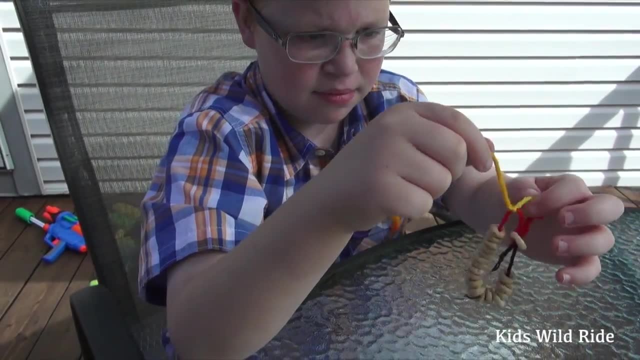 And put these on him. Nice, secure knot. He's got a string. Give us the Cheerios Looking good. Okay, Let's go find a tree guys. Okay, Let's go find a tree guys. Well, those two trees out there look good. 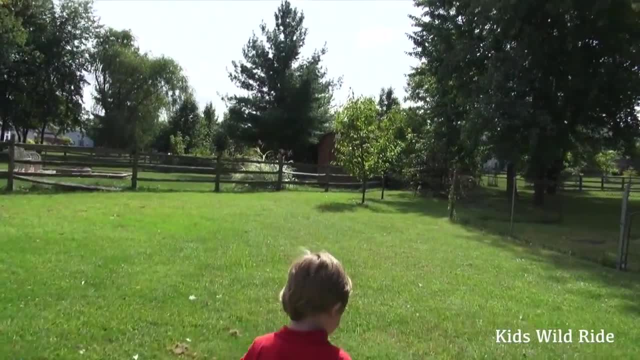 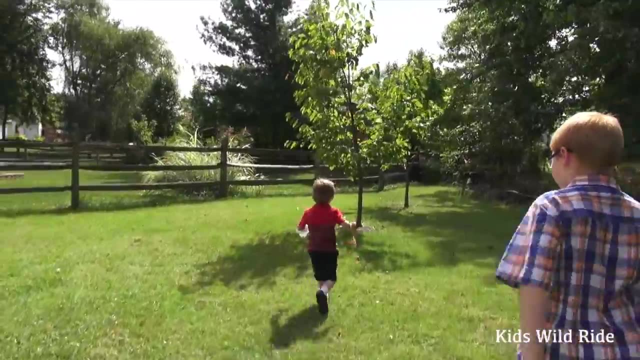 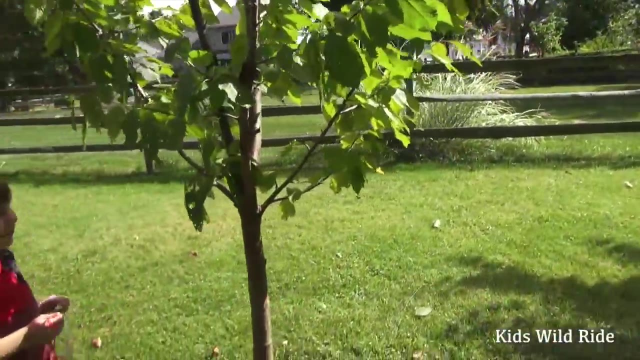 Well, those two trees out there look good. Yeah, we have a couple trees out here. These are cherry trees that we planted a few years ago. Yeah, we have a couple trees out here. Let's try to find a big branch so the branch doesn't break. 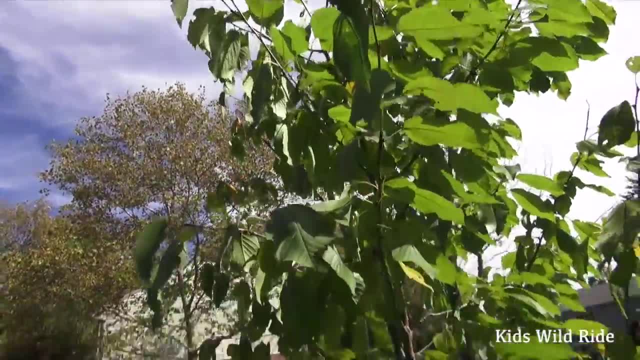 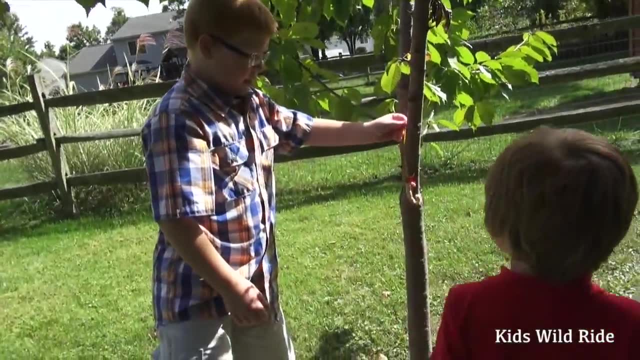 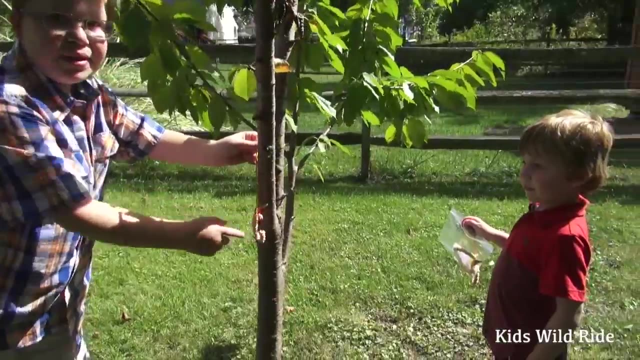 So we have two cherry trees. Let me get out this one. Hold on, I think maybe right here would be fine, because you'd be hanging down from there and then maybe a bird or a squirrel could get up here to eat some. That's a possibility. 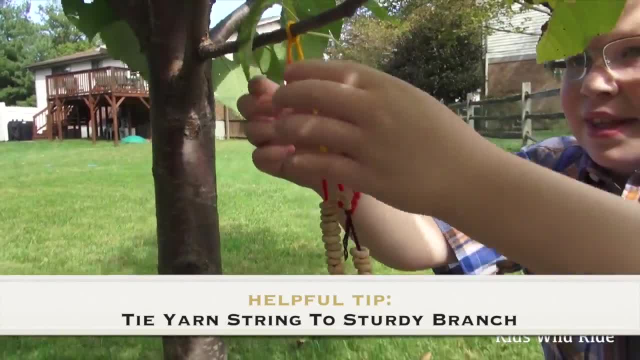 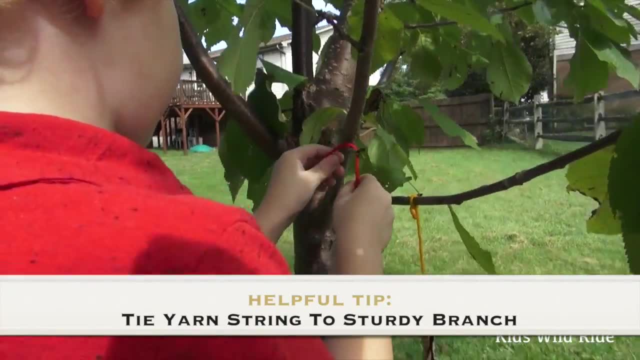 So this is it. This is going to be the final resting spot of our Cheerio bird feeders. Owen's got his attached. We'll double knot it up in a minute here. Liam will help you get yours on too, Looking good. 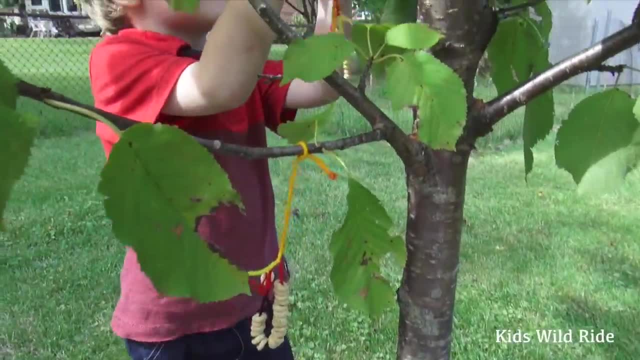 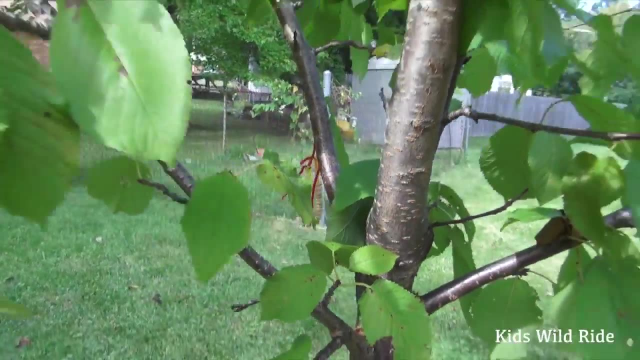 Looking good, So we'll see what happens. Hope you enjoyed our little how-to bird feeder. There it swings. There's Liam's over there. He's got his attached, Let's see. Oh yeah, We'll secure it on nice and tight.